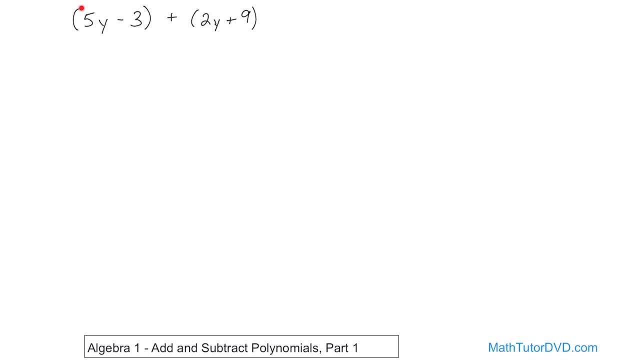 really simplify this anymore or this anymore, So you can kind of mentally drop these together. You can kind of mentally drop these together, So you can kind of mentally the set of parentheses that are surrounding them. Ultimately, you can either mentally do that or you can actually write it down that way, And so let's just show you You could drop it and 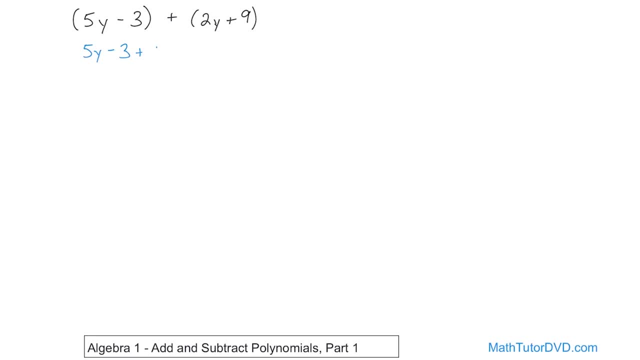 say 5y minus 3 plus 2y minus, I'm sorry- 2y plus 9.. And so these two problems are effectively the same. We were able to drop the parentheses here because effectively you can't do anything further in there. Same thing there as well, And when you drop the parentheses it's a little bit easier to. 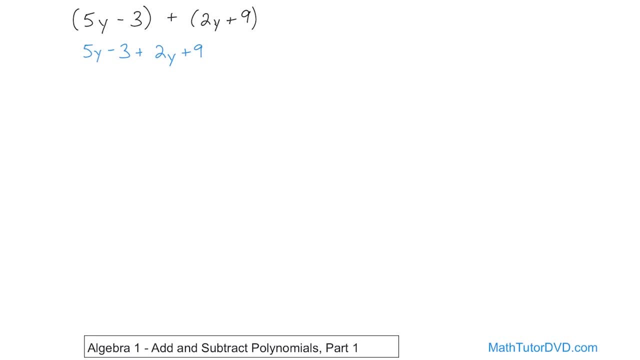 see what you need to do. We're looking at the set of parentheses and we're looking at the set of parentheses and we're looking and hunting around for like terms. Here we have 5y. here we have 2y. 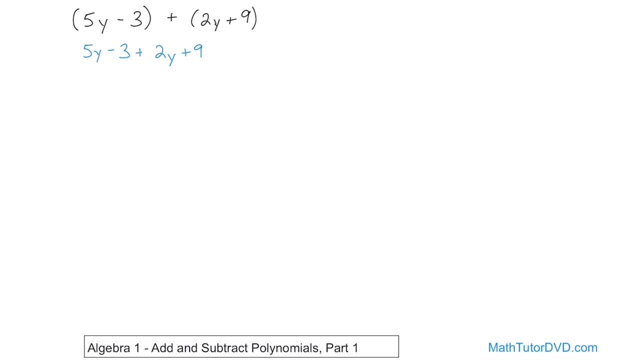 Remember, terms are like: if they contain the same variables, right, So this has a y and this has a y, And they both have numbers in front, so we're able to add those numbers, because they're both talking about the same variable, So we can add them. What is 5 plus 2?? By the way, don't let 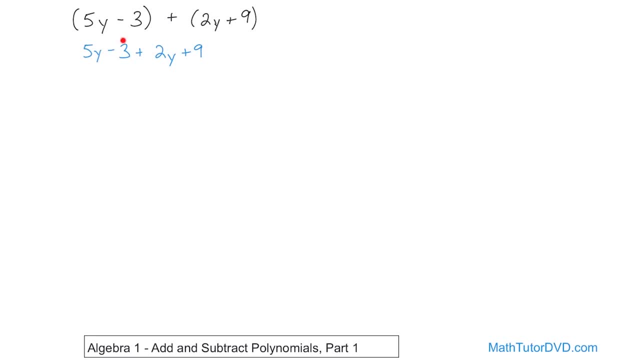 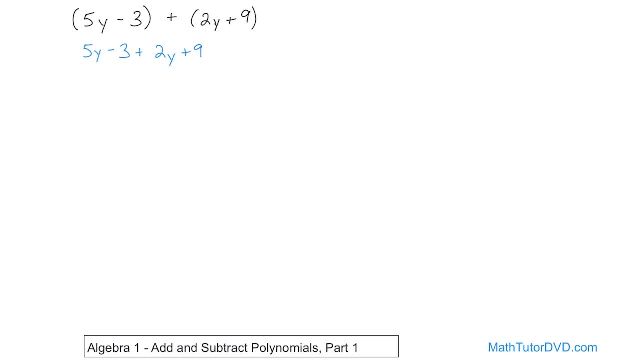 is a positive 2y. So we add them together. normally 5 plus 2 is 7.. So what you're going to get is 7y. Don't forget, the variable has to come along for the ride. It's like 5 jelly beans and. 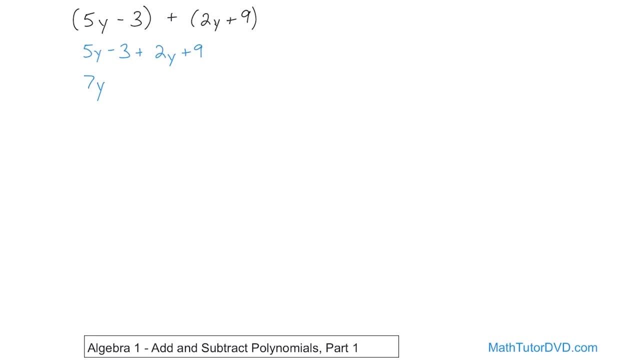 2 jelly beans. You add them together, you get 7 jelly beans. So the variable comes along for the ride. Then you start looking for other like terms. You have a negative 3, and you have a positive 9.. There's no variable associated with either any of those. So those are just numbers. So, of course, 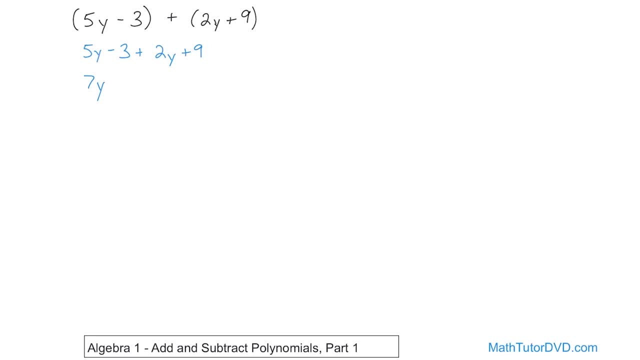 you can add them together. What is negative? 3 plus 9?? The way you handle that is by subtraction: 9 minus 3 is 6. And the sign goes with the larger absolute value, which is 9.. So it's going to be a plus sign. So the answer to this is 7y plus 6.. So congratulations, you've added. 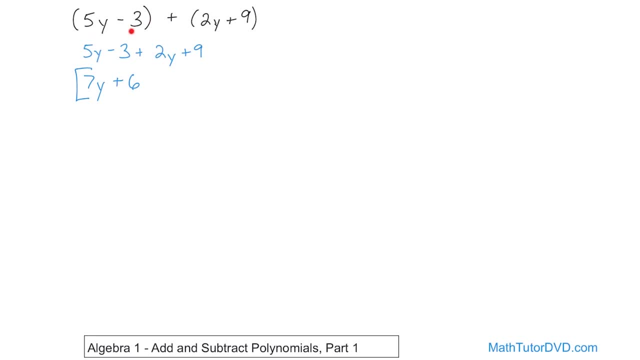 together two polynomials. This is a binomial because it has two terms. This is a binomial because it has two terms And we just added them together. So every problem we do is going to be like this: You're going to look for like terms and you're going to add them together And that's. 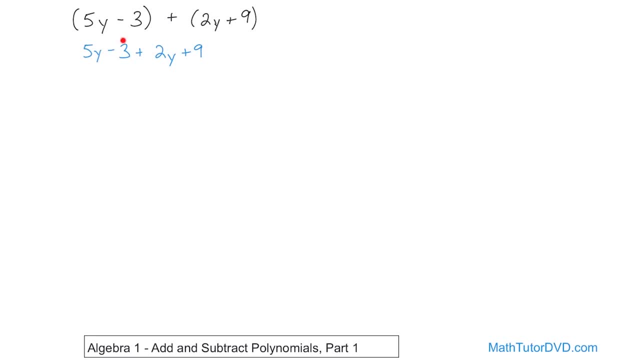 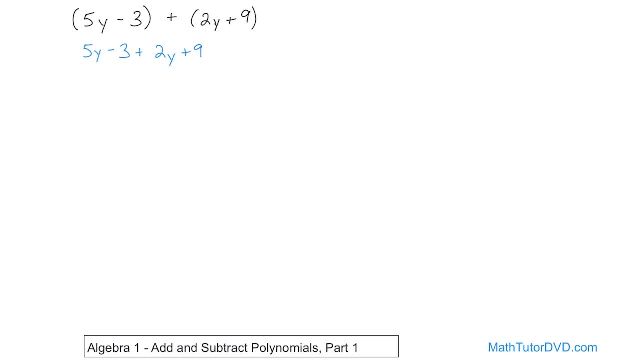 is a positive 2y. So we add them together. normally 5 plus 2 is 7.. So what you're going to get is 7y. Don't forget, the variable has to come along for the ride. It's like 5 jelly beans and. 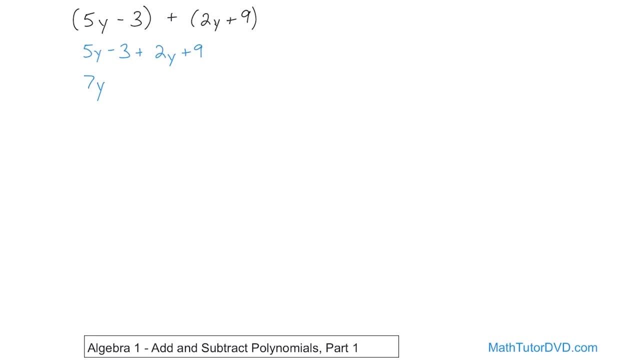 2 jelly beans. You add them together, you get 7 jelly beans. So the variable comes along for the ride. Then you start looking for other like terms. You have a negative 3, and you have a positive 9.. There's no variable associated with either any of those. So those are just numbers. So, of course, 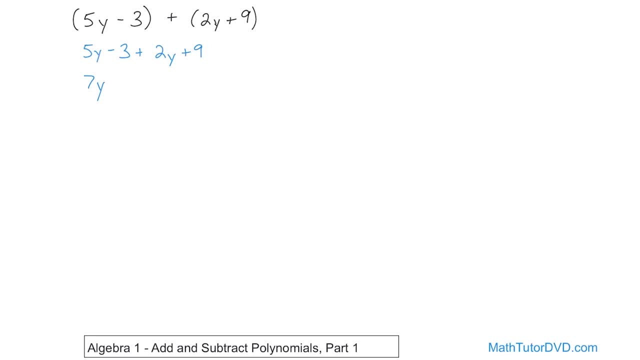 you can add them together. What is negative? 3 plus 9?? The way you handle that is by subtraction: 9 minus 3 is 6. And the sign goes with the larger absolute value, which is 9.. So it's going to be a plus sign. So the answer to this is 7y plus 6.. So congratulations, you've added. 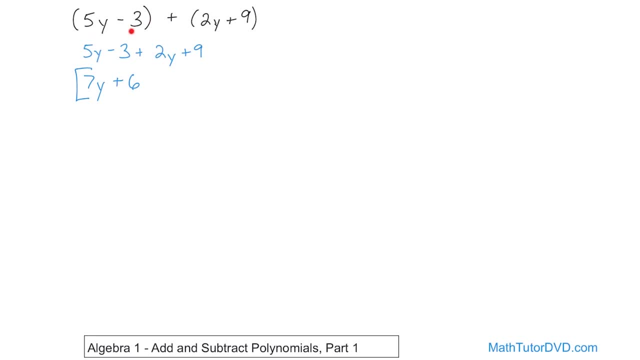 together two polynomials. This is a binomial because it has two terms. This is a binomial because it has two terms And we just added them together. So every problem we do is going to be like this: You're going to look for like terms and you're going to add them together And that's. 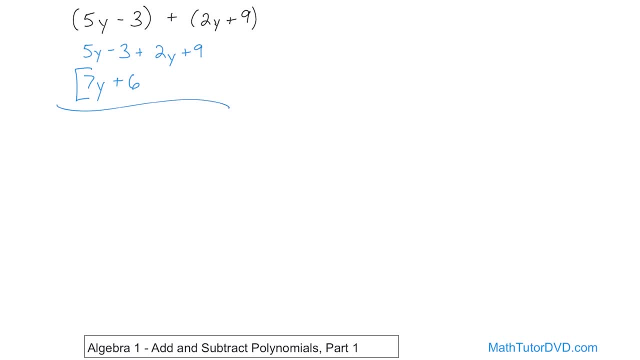 all that there really is to it. So, to take another example, we had, for instance, 3x plus 8. And we're going to add to it 2x minus 5, just like this. So same sort of thing. So you can mentally drop the parentheses if you want, or you could just 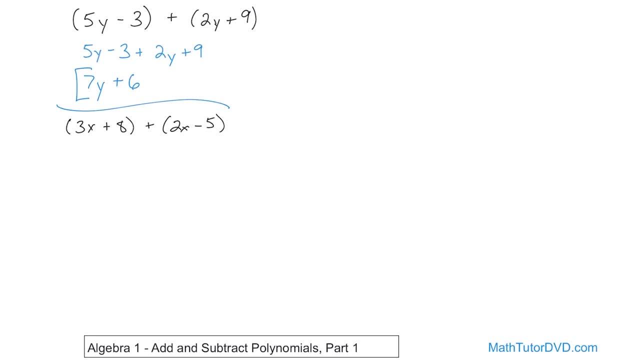 write it all out. And just for the first couple times we'll write it all out. We're able to drop them because there's nothing to do in here. You can't add these together. They're unlike Same thing there, So you can just kind of write it all down: 3x plus 8.. 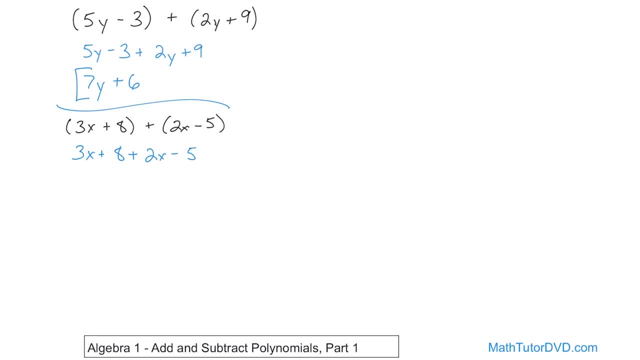 Plus 2x minus 5.. And you don't have to do that, but it sometimes makes it easier to see that you have three x's and two x's. They're both positive, So you can just add them together because they're. 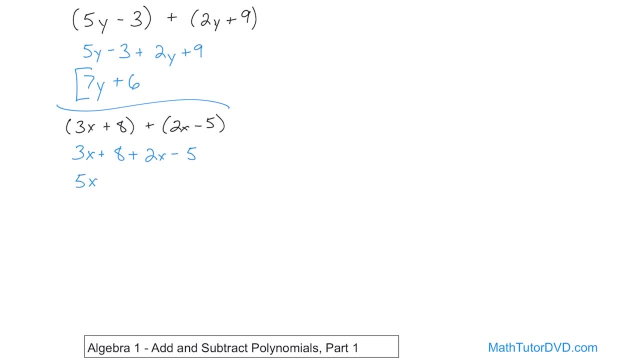 like terms: 3 plus 2 is 5.. So you'll get five x's And then you look, You have 8, and you have negative 5.. So how do you add 8 to negative 5?? Or you can read it as 8 minus 5.. 8 minus 5 is just. 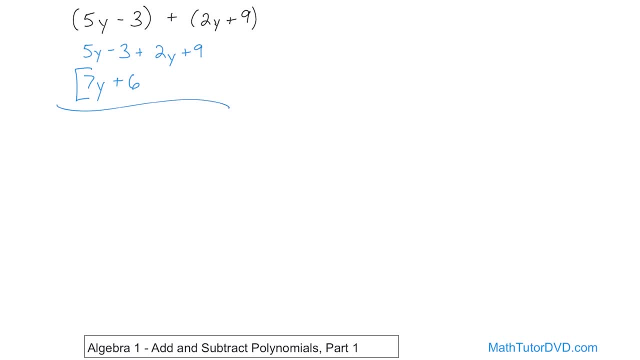 all that there really is to it. So, to take another example, we had, for instance, 3x plus 8. And we're going to add to it 2x minus 5, just like this. So same sort of thing. So you can mentally drop the parentheses if you want, or you could just 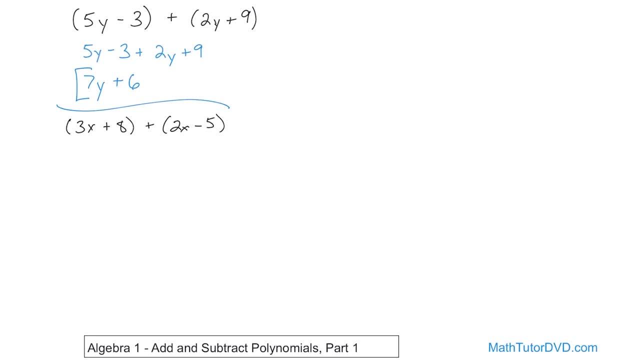 write it all out. And just for the first couple times we'll write it all out. We're able to drop them because there's nothing to do in here. You can't add these together. They're unlike Same thing there, So you can just kind of write it all down: 3x plus 8.. 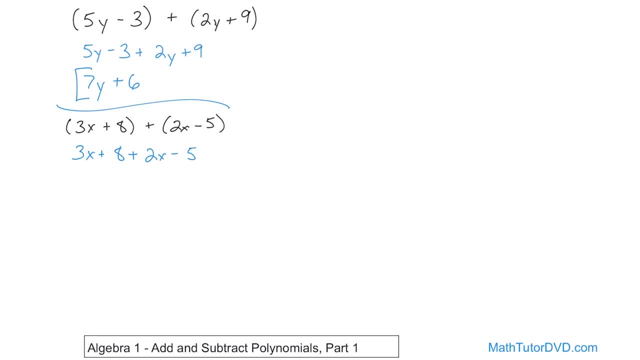 Plus 2x minus 5.. And you don't have to do that, but it sometimes makes it easier to see that you have three x's and two x's. They're both positive, So you can just add them together because they're. 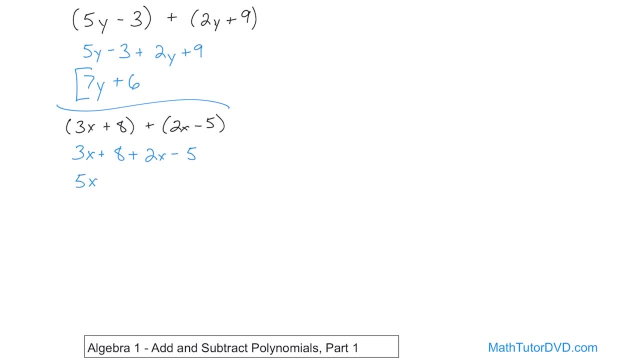 like terms: 3 plus 2 is 5.. So you'll get five x's And then you look, You have 8, and you have negative 5.. So how do you add 8 to negative 5?? Or you can read it as 8 minus 5.. 8 minus 5 is just. 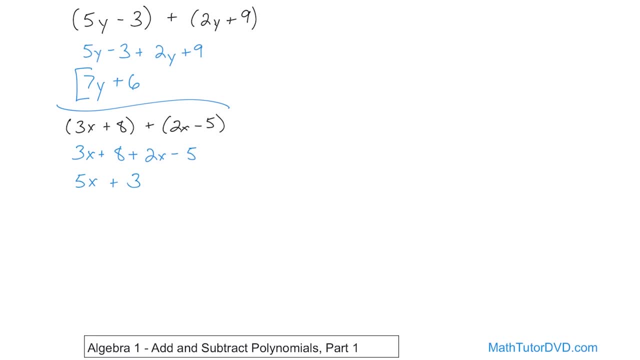 simply 3.. So positive 3.. And the answer is 5x plus 3.. All right, So it's pretty simple. That's what we're going to be doing. You're always going to be hunting for like terms in order to add them. What if you had? let's take something a little bit bigger. 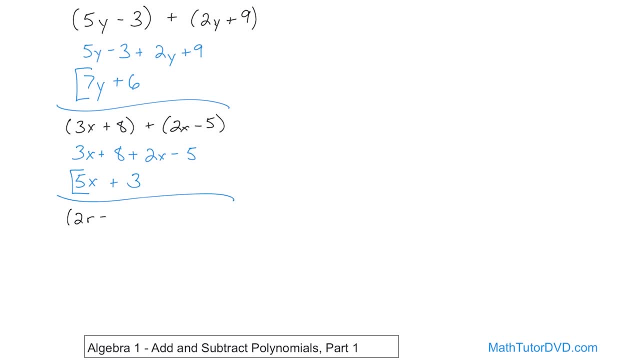 What if you had 2r minus 3x plus 5 plus negative r plus 3x minus 2?? So again we're grouping in parentheses, just showing you that this is a trinomial, So three terms, But notice that the 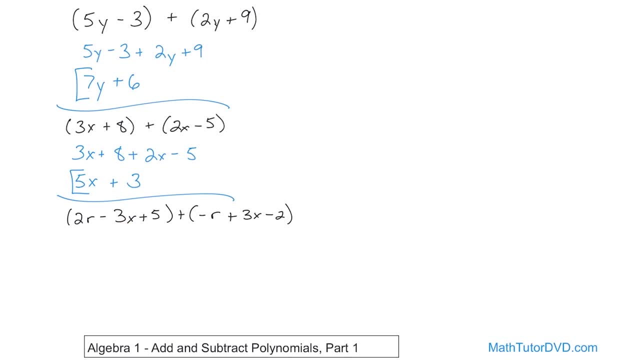 r is an r and the variable here is an x, So these aren't even the same variable And this of course has no variable. And then you have another trinomial rx and then a constant, So you can. 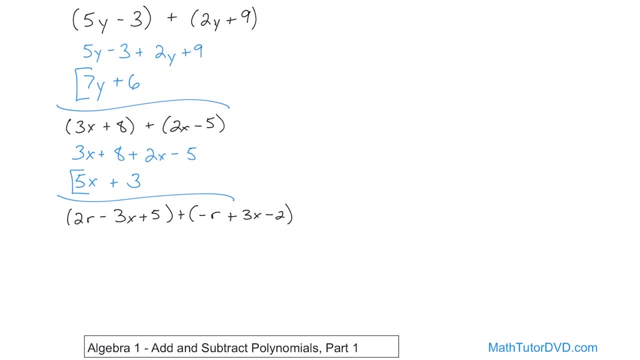 drop the parentheses, because there's nothing to simplify inside of here, And so sometimes it makes it a little easier. So let's do that, And what you'll have here is just 2r minus 3x plus 5.. And then here you've got to be careful, because you have plus, but then you have a negative r, So it's. 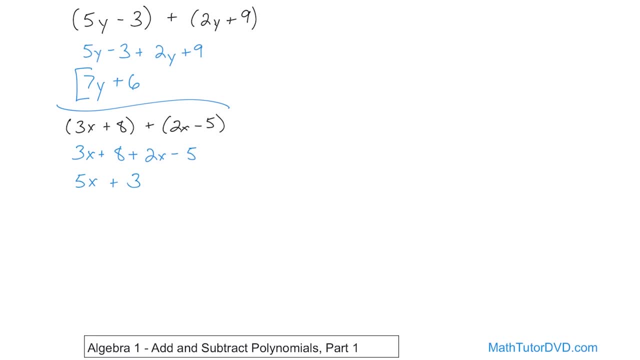 simply 3.. So positive 3.. And the answer is 5x plus 3.. All right, So it's pretty simple. That's what we're going to be doing. You're always going to be hunting for like terms in order to add them. What if you had? let's take something a little bit bigger. 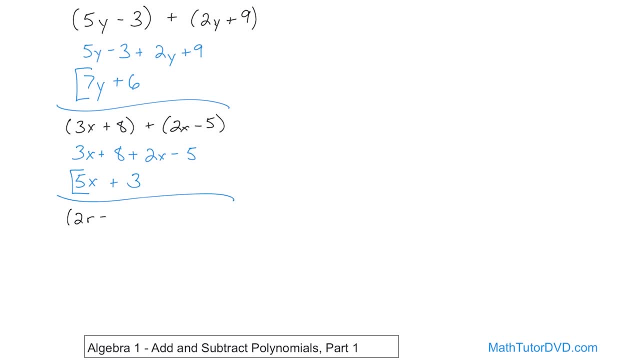 What if you had 2r minus 3x plus 5 plus negative r plus 3x minus 2?? So again we're grouping in parentheses, just showing you that this is a trinomial, So three terms, But notice that the 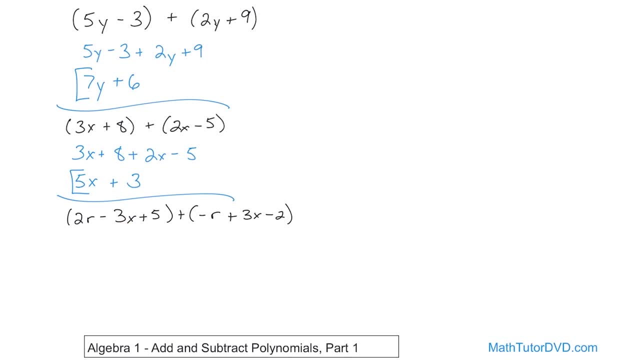 r is an r and the variable here is an x, So these aren't even the same variable And this of course has no variable. And then you have another trinomial rx and then a constant, So you can. 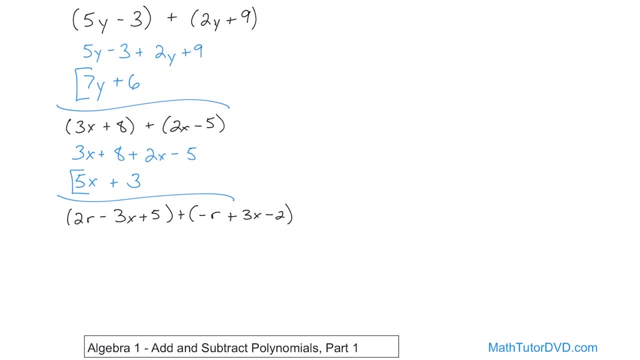 drop the parentheses, because there's nothing to simplify inside of here, And so sometimes it makes it a little easier. So let's do that, And what you'll have here is just 2r minus 3x plus 5.. And then here you've got to be careful, because you have plus, but then you have a negative r, So it's. 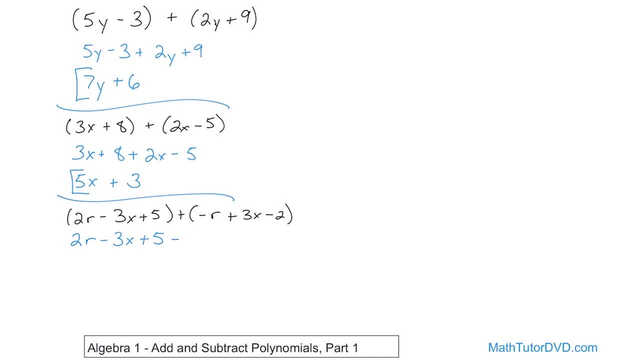 plus negative r, which is going to be written down as just minus, And then you have plus a 3x, So it'll be plus 3x, And then you have plus a minus 2.. So it's going to be written down as just minus 2.. Now you just need to be careful. You could write this as plus negative. 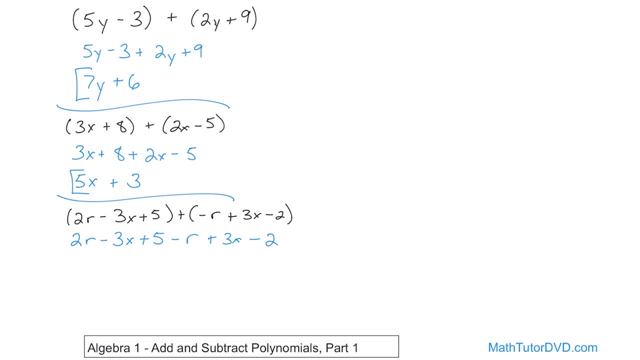 r and you could write this as plus negative 2.. But you all know when you have plus negative something, it's the same thing as subtraction. So when you read it like this, just write it as subtraction here and here. Basically, the signs are coming from inside of there. So now that we 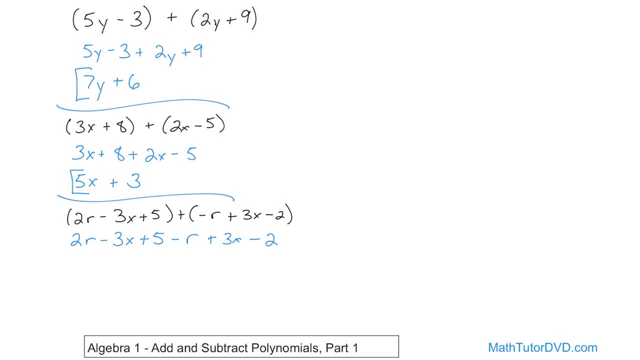 have written down, we start to hunt for these like terms. So we see that we have 2r's positive 2r and here we have negative r. So how do you add those together? You can also read this: 2r minus r. 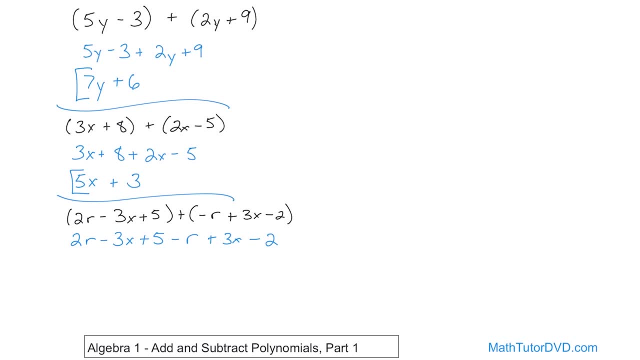 or 2 minus 1.. So that's just going to give you a positive 1 or positive r in this case, because you have to keep the variable. So basically, the subtraction of 2r minus r just simply becomes r or 1r. 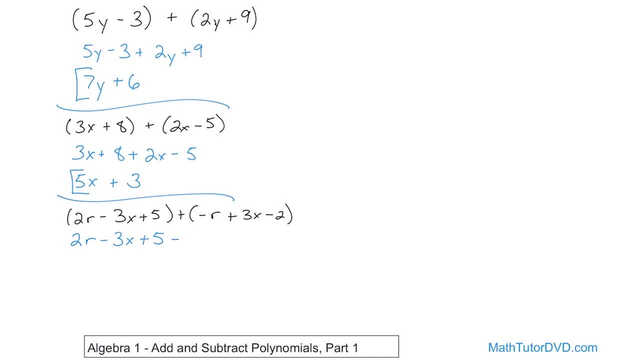 plus negative r, which is going to be written down as just minus, And then you have plus a 3x, So it'll be plus 3x, And then you have plus a minus 2.. So it's going to be written down as just minus 2.. Now you just need to be careful. You could write this as plus negative. 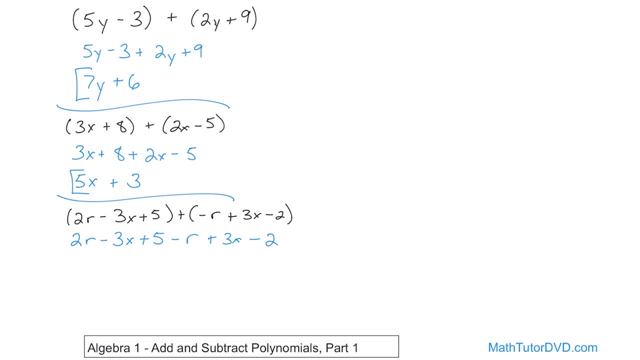 r and you could write this as plus negative 2.. But you all know when you have plus negative something, it's the same thing as subtraction. So when you read it like this, just write it as subtraction here and here. Basically, the signs are coming from inside of there. So now that we 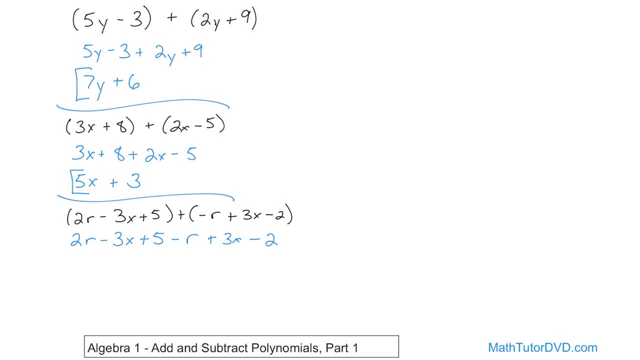 have written down, we start to hunt for these like terms. So we see that we have 2r's positive 2r and here we have negative r. So how do you add those together? You can also read this: 2r minus r. 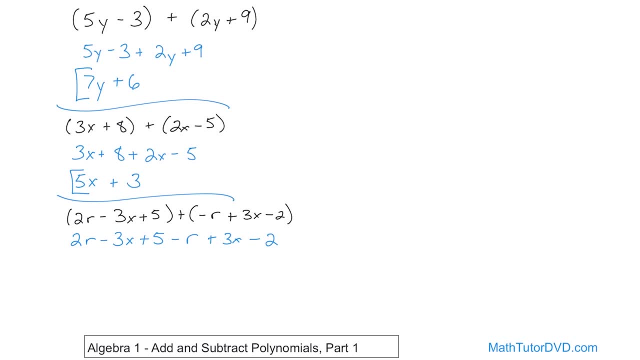 or 2 minus 1.. So that's just going to give you a positive 1 or positive r in this case, because you have to keep the variable. So basically, the subtraction of 2r minus r just simply becomes r or 1r. 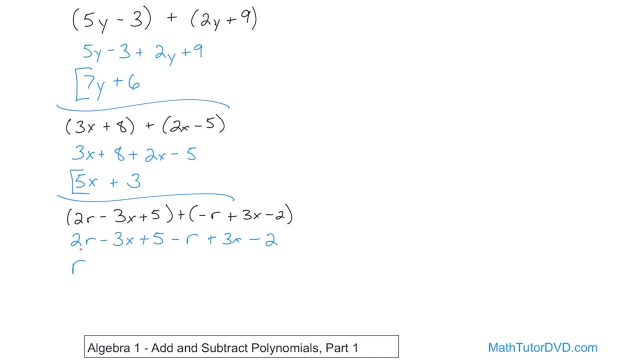 What I like to do when you have lots and lots of terms like this is, after I add things together, I put a little dot underneath it And the dot reminds me that I've already handled those two terms. So now I can go and look at other things and look for other things that are similar. 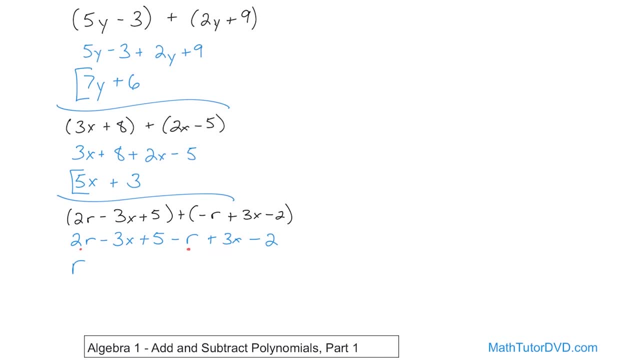 So here I have negative 3x and here I have positive 3x. What's that going to add together to equal Negative 3 plus 3 is going to be 0. So instead of writing 0 down, I'm just going to. 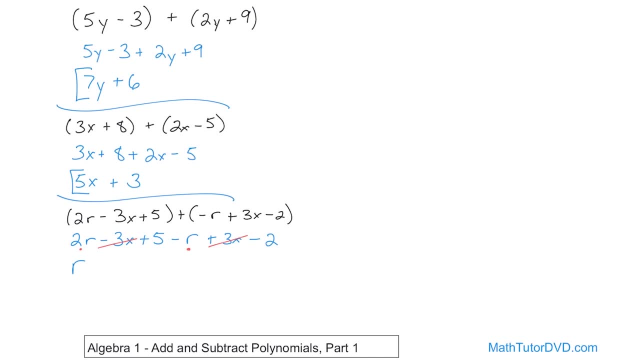 strike through this and strike through this, And that reminds me that they don't really, I guess, vanish into thin air. It's just that they add together To give you 0. So you don't write anything down for those, And here you have 5 minus 2 or 5 plus. 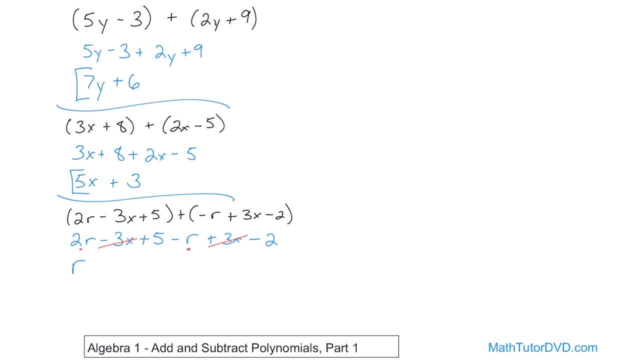 a negative 2, if you want to think of it that way, But it's 5 minus 2, which is going to give you a positive 3.. So we'll go change the color back here and give us positive 3.. So the answer is r. 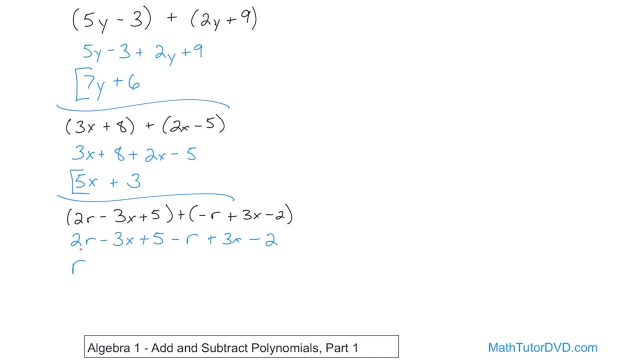 What I like to do when you have lots and lots of terms like this is, after I add things together, I put a little dot underneath it And the dot reminds me that I've already handled those two terms. So now I can go and look at other things and look for other things that are similar. 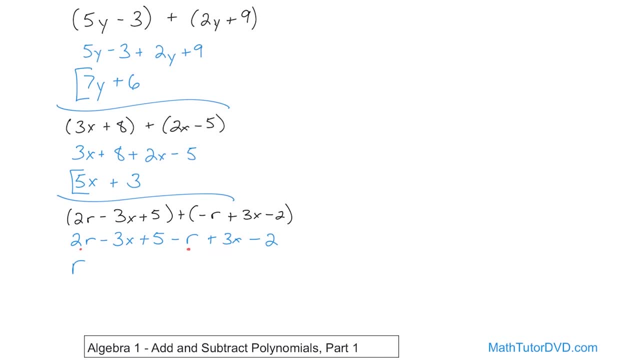 So here I have negative 3x and here I have positive 3x. What's that going to add together to equal Negative 3 plus 3 is going to be 0. So instead of writing 0 down, I'm just going to. 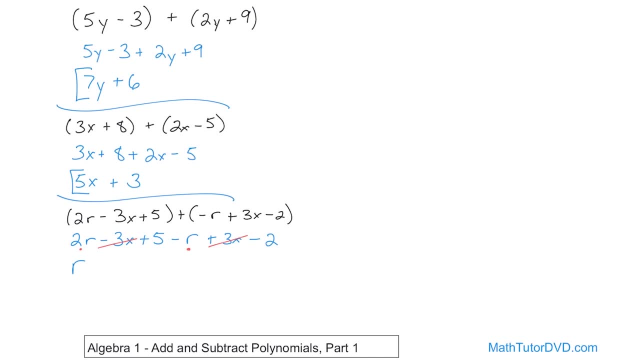 strike through this and strike through this, And that reminds me that they don't really, I guess, vanish into thin air. It's just that they add together To give you 0. So you don't write anything down for those, And here you have 5 minus 2 or 5 plus. 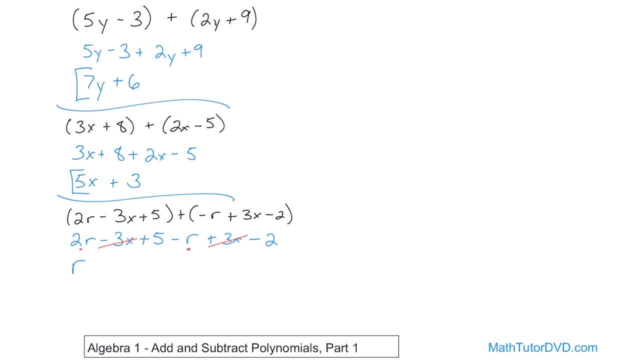 a negative 2, if you want to think of it that way, But it's 5 minus 2, which is going to give you a positive 3.. So we'll go change the color back here and give us positive 3.. So the answer is r. 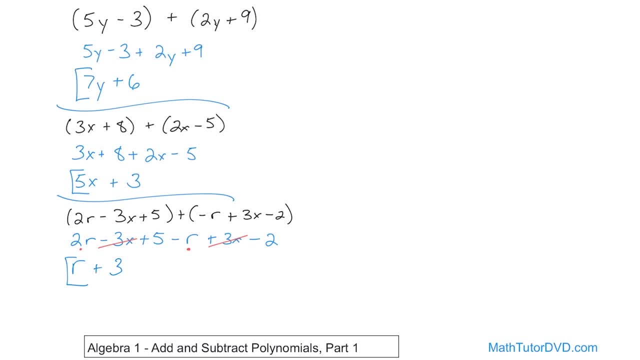 plus 3.. That's the final answer. So again, you just write everything down, look for these like terms and then go to town trying to simplify them. What if you have 2x minus 5, minus x minus 2? Now here's our first problem where we're subtracting polynomials. You see here 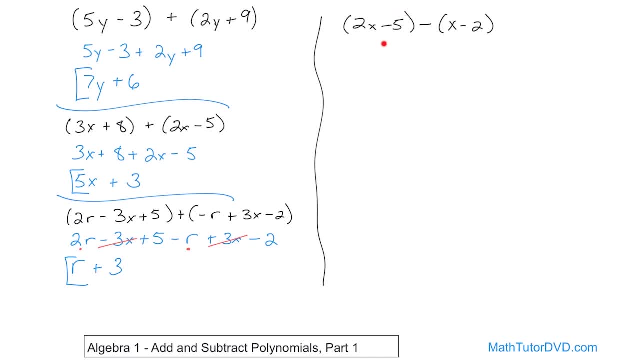 we were adding polynomials together in all three cases. Here we have a polynomial- a binomial in this case- and we're subtracting from it another binomial. So here you do have to be careful, because you have this minus sign. So you really do need to write everything down before you try. 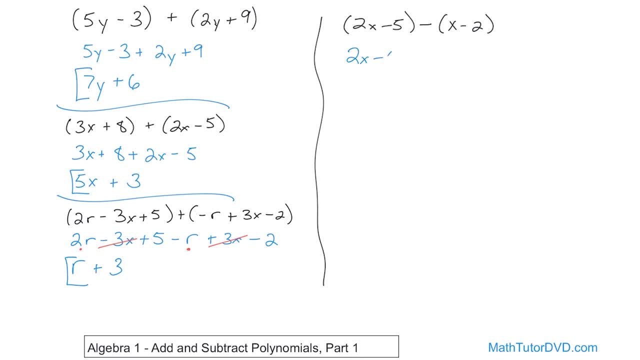 to do the subtraction. So, for instance, you're going to have 2x minus 5. We can drop those parentheses, But here you see this negative. it's really a negative 1 out here. You need to distribute it into here and distribute it into there. Remember that distributive property I told. 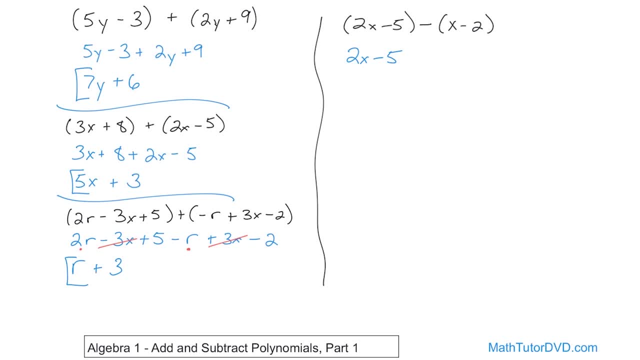 you that you'd be using it over and over again, and you will be, So this is going to be written as minus x. Let me switch back here. Minus x, And what do you think is going to happen when you distribute the negative in here? It's like negative 1 times negative 2.. So you're going to 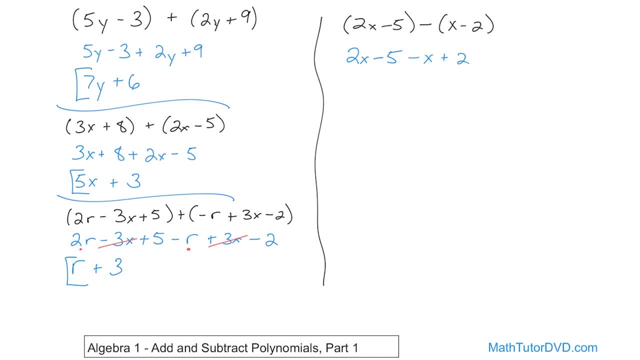 get a positive 2.. So when you distribute the negative in here you get negative x. Distribute here It changes it to a positive 2 because of the rules of multiplication in algebra. So now you start looking for like terms. You have positive 2x minus x or you can read it as 2 minus 1 because there's an implied 1 here. 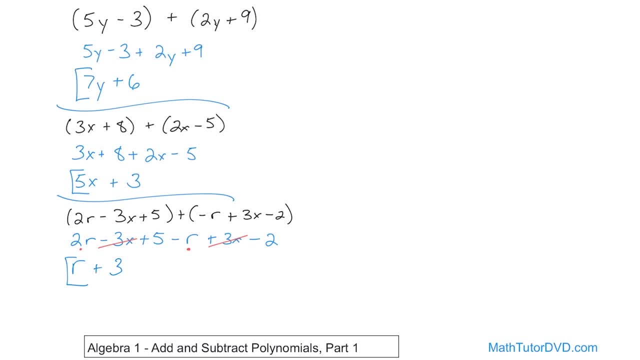 plus 3.. That's the final answer. So again, you just write everything down, look for these like terms and then go to town trying to simplify them. What if you have 2x minus 5, minus x minus 2? Now here's our first problem where we're subtracting polynomials. You see here 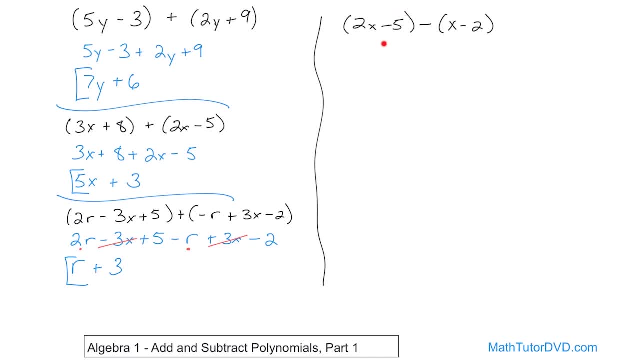 we were adding polynomials together in all three cases. Here we have a polynomial- a binomial in this case- and we're subtracting from it another binomial. So here you do have to be careful, because you have this minus sign. So you really do need to write everything down before you try. 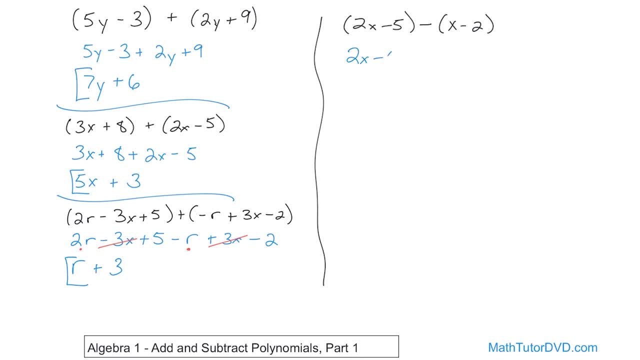 to do the subtraction. So, for instance, you're going to have 2x minus 5. We can drop those parentheses, But here you see this negative. it's really a negative 1 out here. You need to distribute it into here and distribute it into there. Remember that distributive property I told. 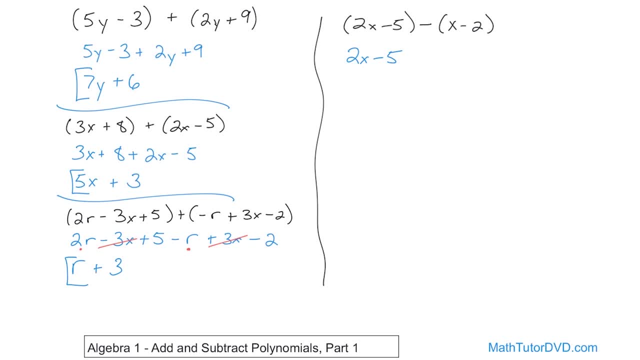 you that you'd be using it over and over again, and you will be, So this is going to be written as minus x. Let me switch back here. Minus x, And what do you think is going to happen when you distribute the negative in here? It's like negative 1 times negative 2.. So you're going to 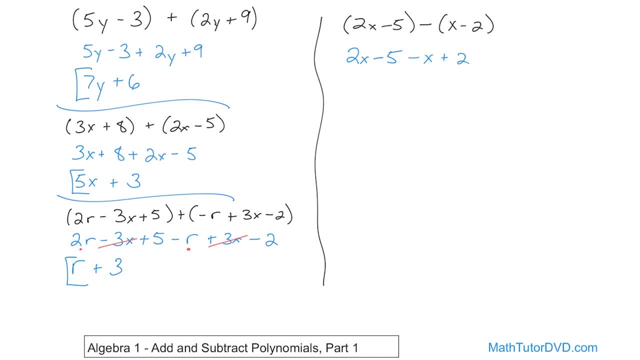 get a positive 2.. So when you distribute the negative in here you get negative x. Distribute here It changes it to a positive 2 because of the rules of multiplication in algebra. So now you start looking for like terms. You have positive 2x minus x or you can read it as 2 minus 1 because there's an implied 1 here. 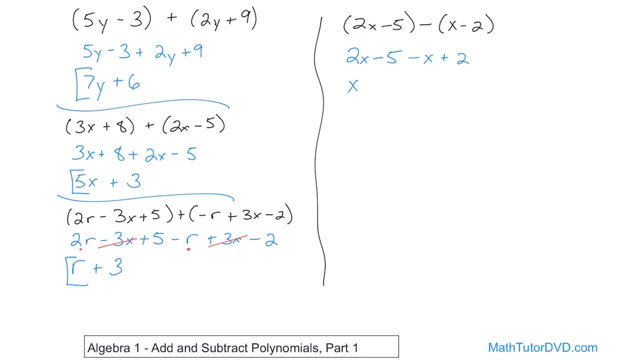 2 minus 1 is 1.. And of course you still have to keep the x, So it's going to be x. And then you have negative 5 plus 2.. How do you handle that? Well, you subtract: 5 minus 2 is 3.. And the sign: 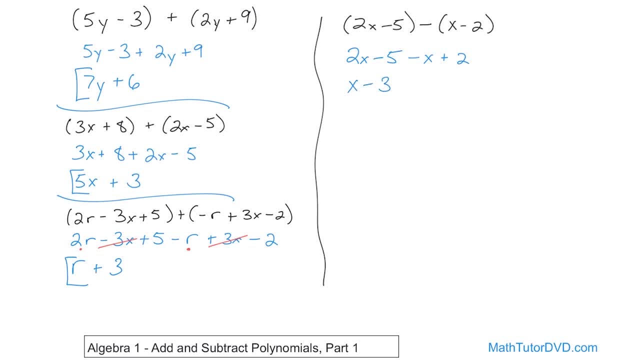 goes with the larger absolute value, which is negative 5.. So it's going to be x minus 3.. And that's the final answer. You have to be really careful when you're subtracting polynomials to get the correct sign so that you can add everything together. All right, So this will be our final. 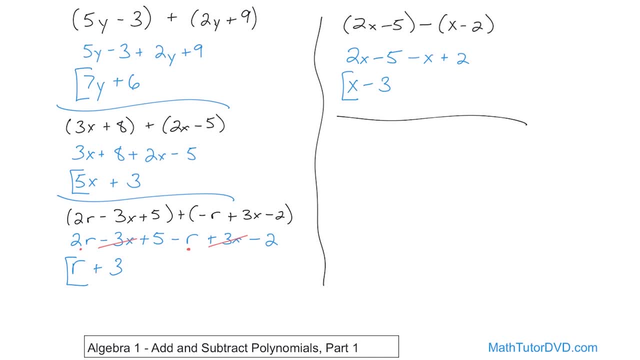 lesson, or our final question in this lesson: What if we had 5x minus 3t minus 7? And we're subtracting from that x minus 2t minus 3.. All right, So now we have the same sort of thing. 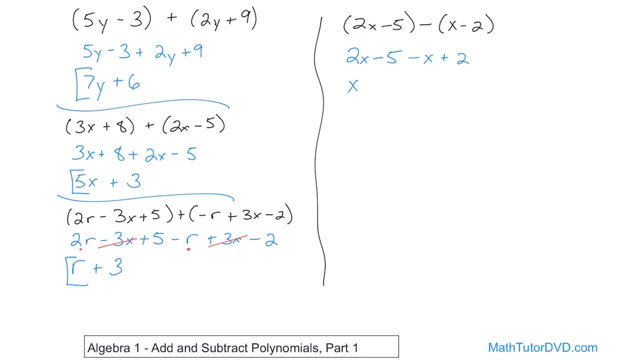 2 minus 1 is 1.. And of course you still have to keep the x, So it's going to be x. And then you have negative 5 plus 2.. How do you handle that? Well, you subtract: 5 minus 2 is 3.. And the sign: 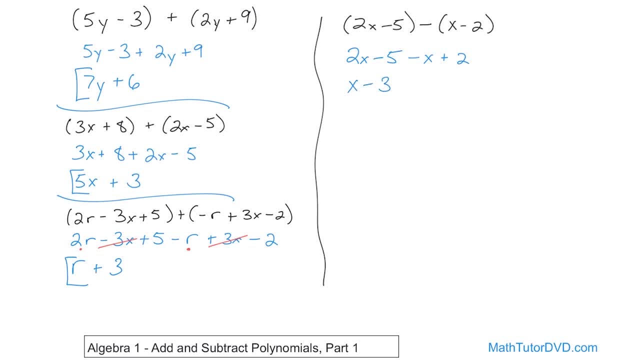 goes with the larger absolute value, which is negative 5.. So it's going to be x minus 3.. And that's the final answer. You have to be really careful when you're subtracting polynomials to get the correct sign so that you can add everything together. All right, So this will be our final. 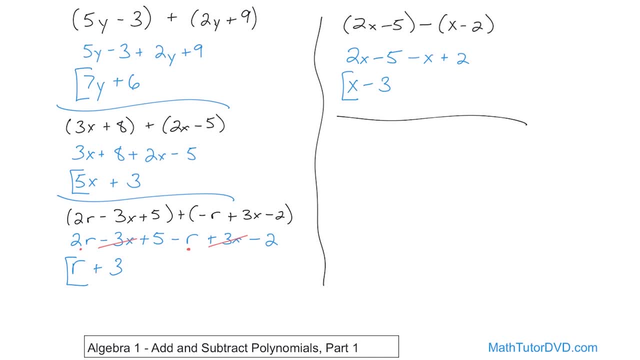 lesson, or our final question in this lesson: What if we had 5x minus 3t minus 7? And we're subtracting from that x minus 2t minus 3.. All right, So now we have the same sort of thing. 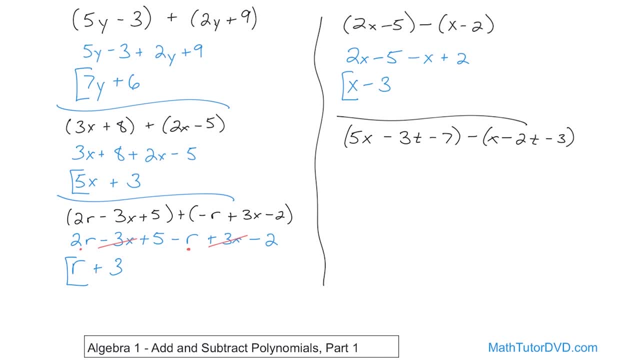 You have two variables, an x and a t, and then of course nothing here, And you're subtracting another trinomial, also with x's, t's and a constant. So you need to really write everything down and distribute that negative in there. So you're going to have 5x minus 3t. We're just 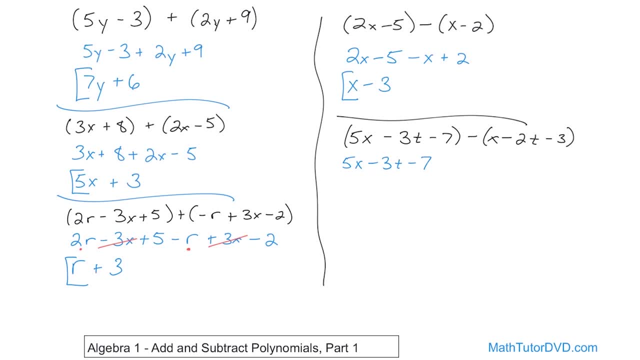 dropping the parentheses here because there's nothing else we can do inside. We can't actually add those things together And we distribute this negative 1. That's going to make that negative x. And then when you distribute to the negative times negative, it's going to give you positive 2t. 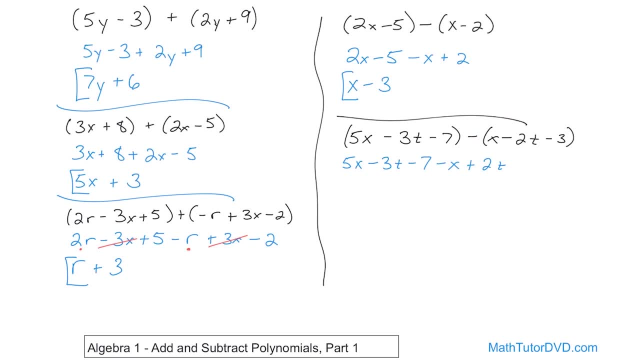 And then the same thing is going to happen here: Negative times, negative 3, is going to give you negative 3.. So now we can start hunting for like terms. We have a 5x and we have a minus x, So this is 5 minus 1, which is going to give you 4x, And I'm going to go ahead and put a dot under this. 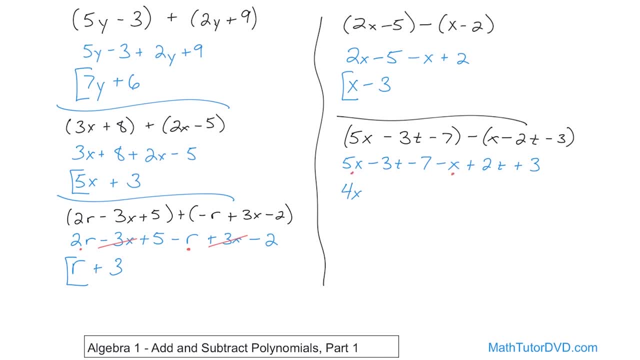 and under this to remind myself that I've handled it. And then I'm going to look over here at negative 3t plus t, Or you can read it as negative 3 plus 2. How do you handle that? You subtract them And the sign is going to go with a larger absolute value, So it's going to be negative. 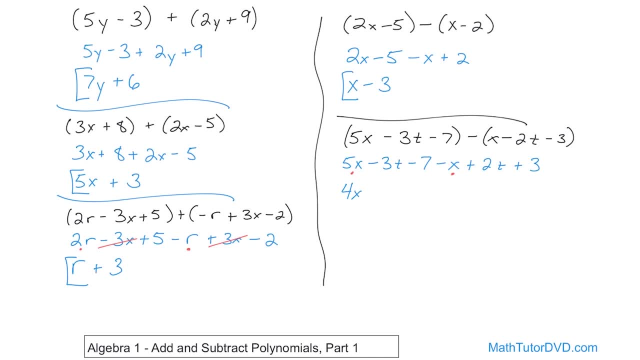 Let me change colors. It's going to be negative 1t. So it's going to be negative t Because 3 minus 2 is 1. And the sign goes with a larger absolute value. So you have a negative sign And the t comes from the fact that